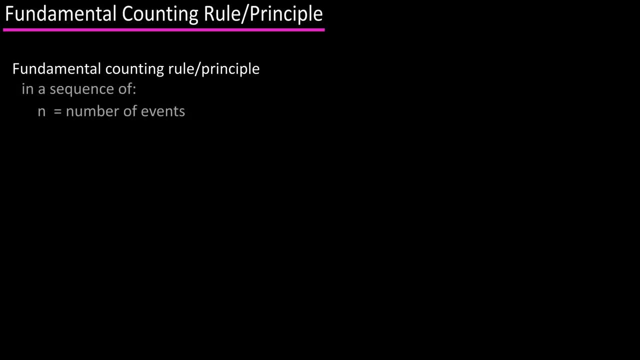 rule or principle which mathematically says: in a sequence of n number of events, where the first event has k1 number of possibilities and the second event has k2 number of possibilities and so on, the total number of possibilities of the sequence will be: 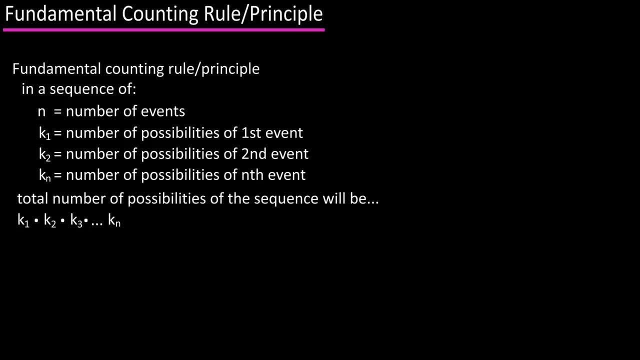 k1 times k2 times k3 times. dot, dot, dot kn. What this is saying in simpler terms is that when you have a certain number of events, like in our example, shirts, shorts and shoes, to find the total amount of possibilities of the sequence you have to multiply the total number of possibilities. 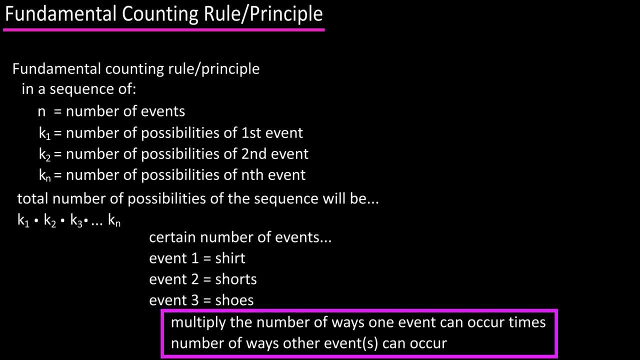 of the sequence. You multiply the number of ways one event can occur times the number of ways the other events can occur. So seven different colors for the shirt, four different colors for the shorts and five different colors for the shoes. When we multiply them together, seven times four. 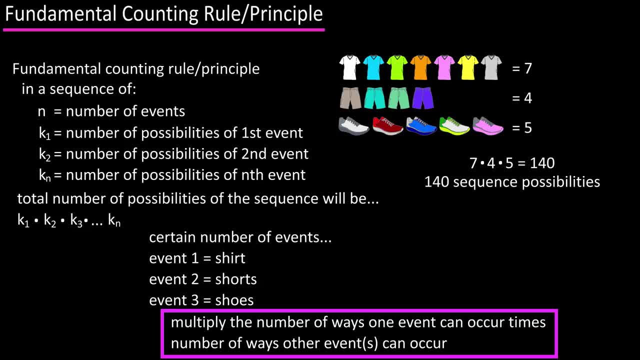 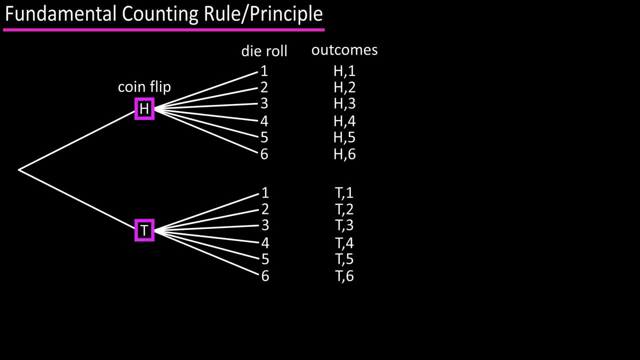 times five, we get 140 possibilities of the sequence. To show this visually, here is a tree diagram for a coin flip and a die roll. You can have a head or a tail on the coin flip and a one through six on the die roll. As you can see on the right, there are 12 possible outcomes. 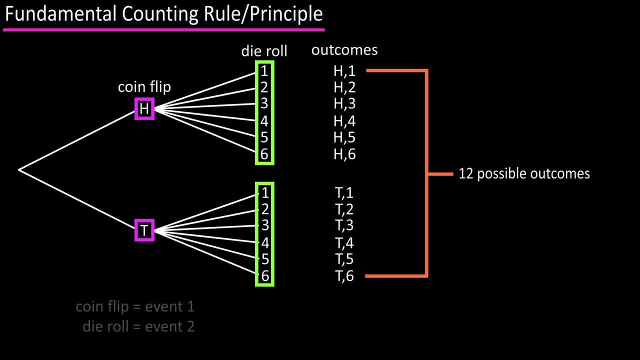 Using the fundamental counting rule, with the coin flip as event one and the die roll as event two, we have two possibilities for the coin flip and six for the die roll. So two times six equals 12.. Same result as the tree diagram. One more example is a four number pin code for a credit card. 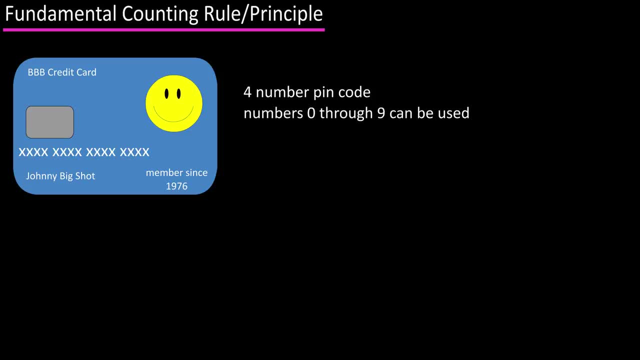 Numbers zero through nine can be used. So four number code means four events and zero through nine means 10 possibilities for each event. 10 times 10 times 10 times 10 equals 10,000. So 10,000 possibilities of the sequence. All right, my friends, hopefully this video helped you out. 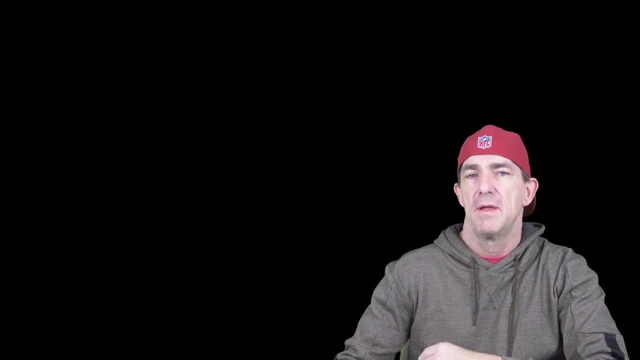 I do have more videos right there for you Till next time I am out of here.